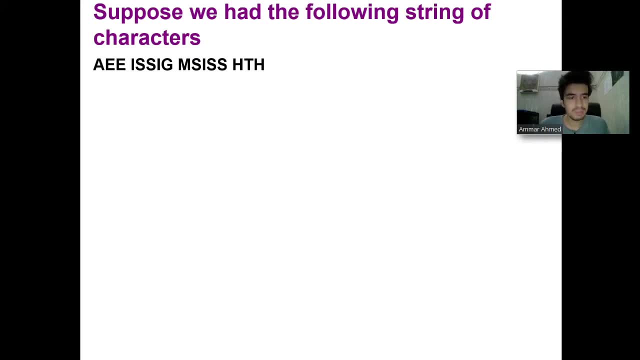 we have. suppose we have a string of characters. What we are doing is that, taking a file as an input, a text file as an input, and the whole goal is to reduce the file size. So suppose we have a string of characters and we want to somehow reduce its size Initially. 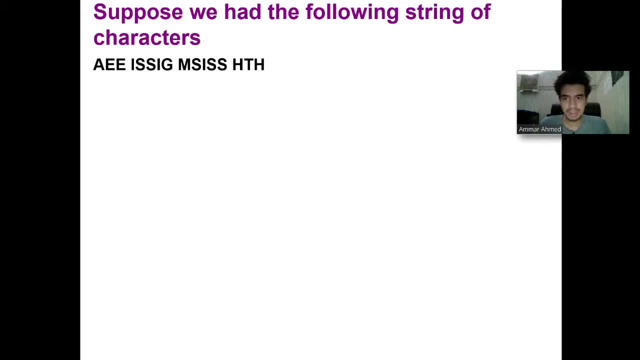 if you think about it, that each character is represented with 8 bits using ASCII, So suppose it is represented by this list of 8 bits. Likewise, E, all the way up to: so these are all the distinct characters that are in this string, in this following string right here: 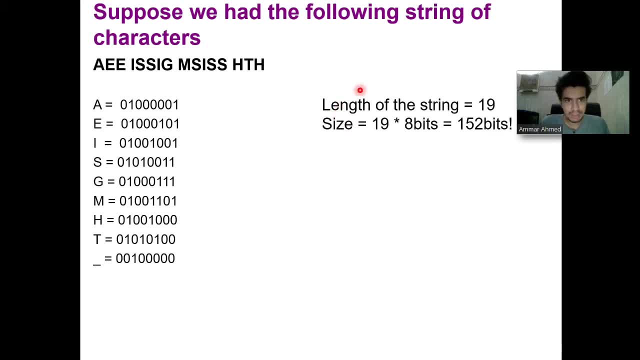 Now, if I look at the length of this string, I see that its length is 19 and if I multiply 19 by 8 I get 152 bits. So the total size of this string is 152 bits. That means, if I want to say 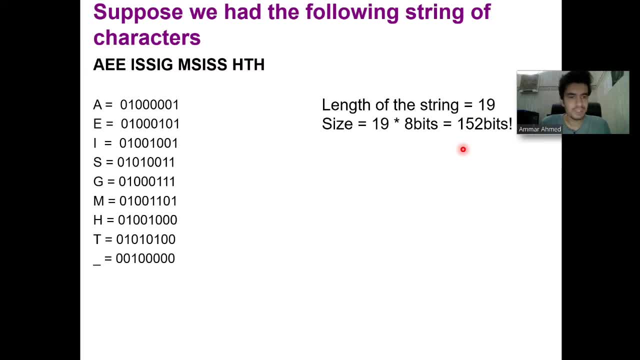 that I want to send this string over a network or I want to store this string somewhere, I require at least 152 bits, So how can we reduce the size of this string? Essentially, if we answer this question, we can also reduce the size of the file that contains the text. 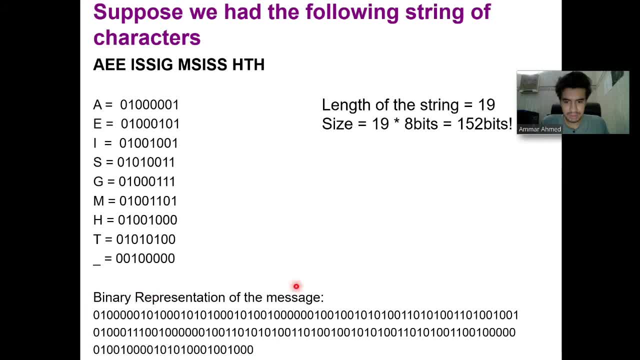 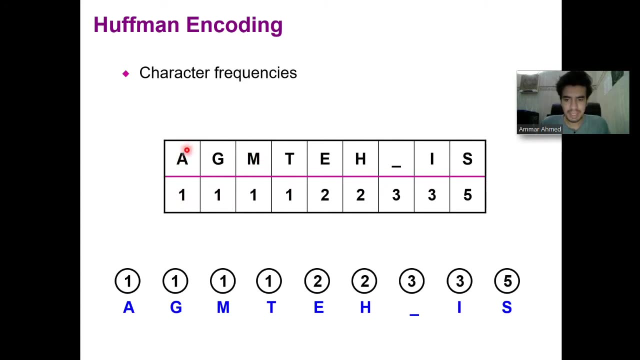 So you can see the binary representation of the message below here. So this represents all of these characters. In other words, if you look at this string, you can see that there are 5 bits in it. So these are the distinct characters in their bit sequence respectively: Okay, so these 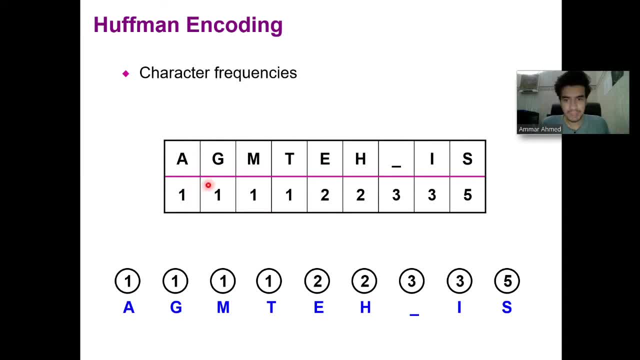 are the character frequencies, meaning that A has appeared only one times in the previous string and S has appeared five times, right? So these are the distinct characters and their frequencies, In other words, how many times each character have occurred in a string. 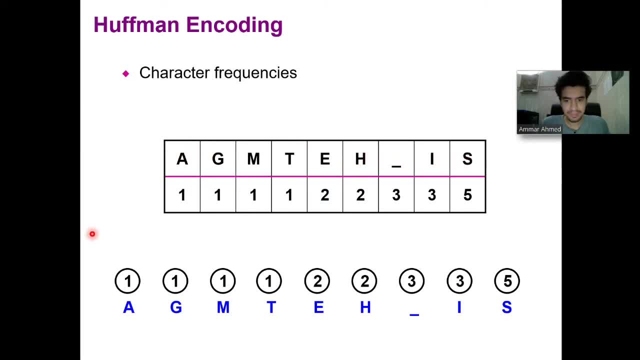 So what Huffman says, or Huffman Coding says, is that create the nodes for each of these distinct characters in their bit sequence, In other words, how many times each character has occurred in a string. So what Huffman says is that create the nodes for each of these distinct characters in their 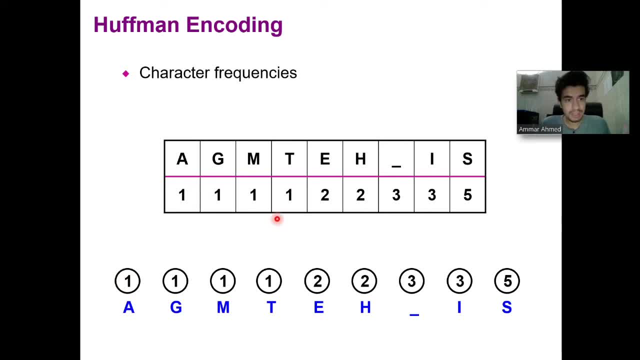 bit sequence, And each node should have the following properties: a character and its frequency. So we have created these, you know these, uh nine nodes, right, Uh, A, G, M, T, right, Each of which contain their frequencies And what Huffman says. that okay. 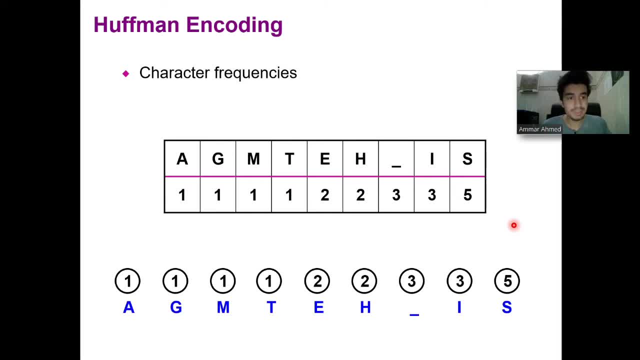 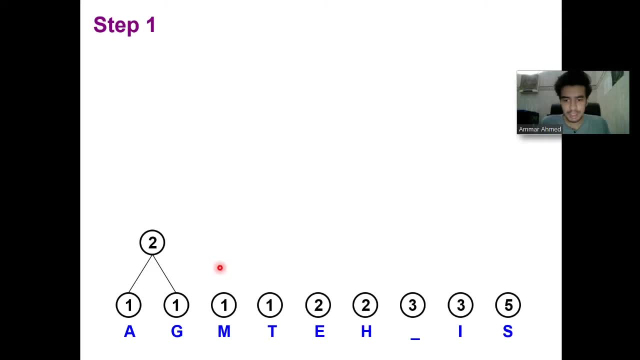 now combine those nodes that have the least frequency, frequency. So you have to combine two nodes with the least frequency. So if we do that, we combine first A and G to get a node with frequency two, the, in other words some of 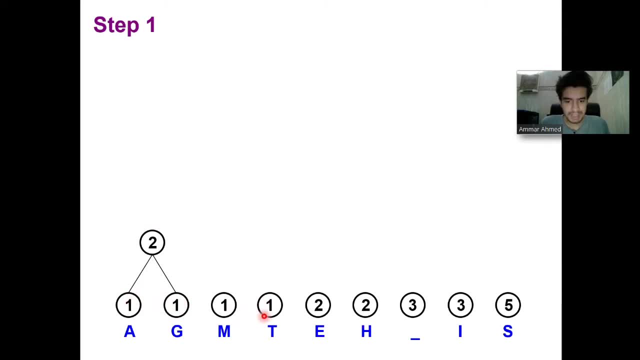 these two nodes. if we combine now M and D, because these are the next least two uh nodes that have least frequency, we get two. Now we combine these two. You could also combine these two, but I'm going to combine these two to get four. Now the least uh nodes. 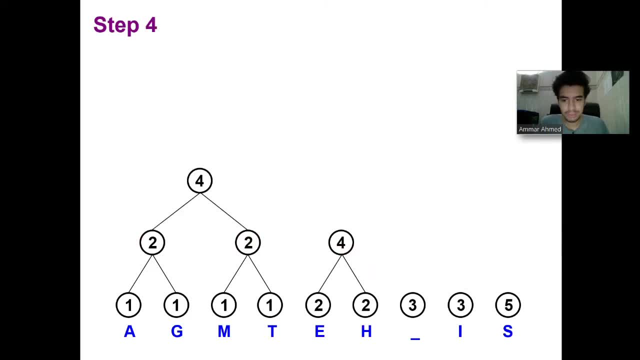 right now the least two nodes are two and two. So if we combine these two, we're going to combine pick to get six and hide We combine pick to get one. if we rounded up the node length by a thread and the length of друзья and 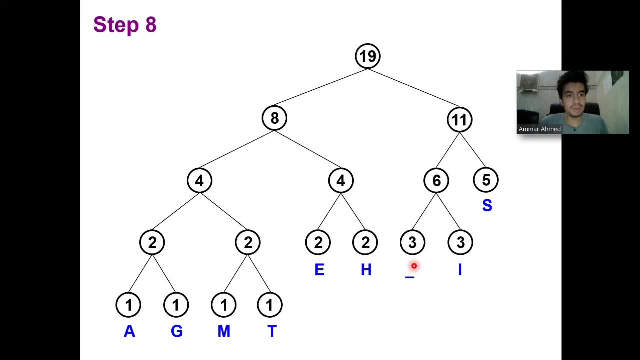 a wheel founded with Uh, two, three, 1 to get ghi, to get three, to get six, which this 19 is a root node, right? so what is the point of creating this tree? you know, if we want to reduce the file size? well, the point is that these edges 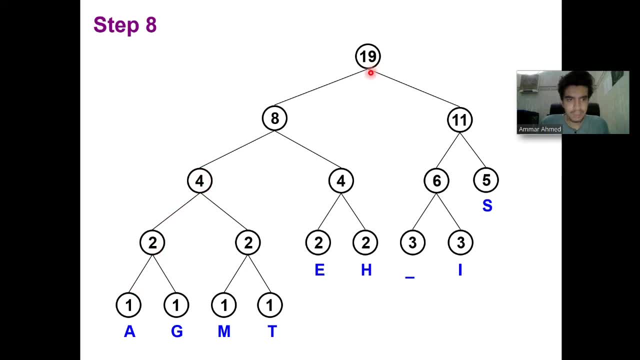 if you see these edges in a tree, right what Huffman says, that we can use these edges to represent the bit sequence of each character. in other words, we can represent A like this: 0 0, 0, 0, so the source code of A, instead of representing A with. 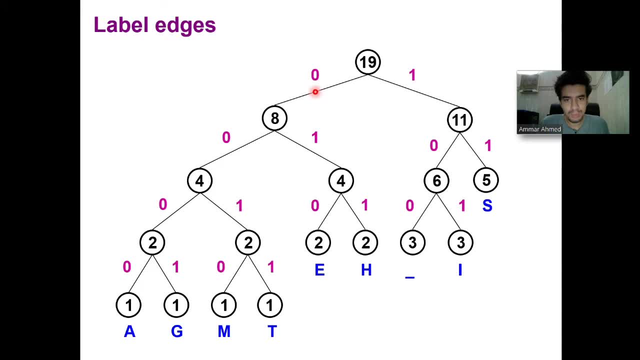 8 bits. we can represent A with this four bits right, essentially 0, 0, 0, 0. and if we are representing, we were to represent H, we can represent H by 0, 1, 1, essentially traversing the tree in this manner. so what Huffman says whenever you: 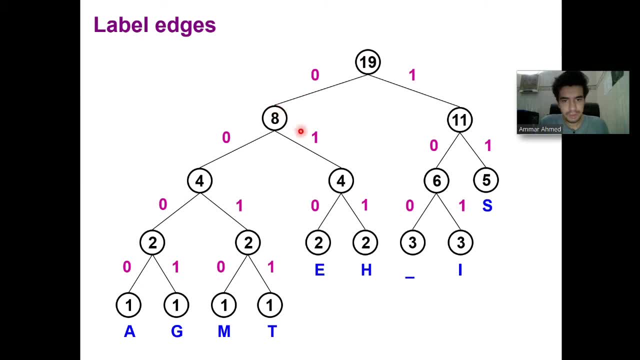 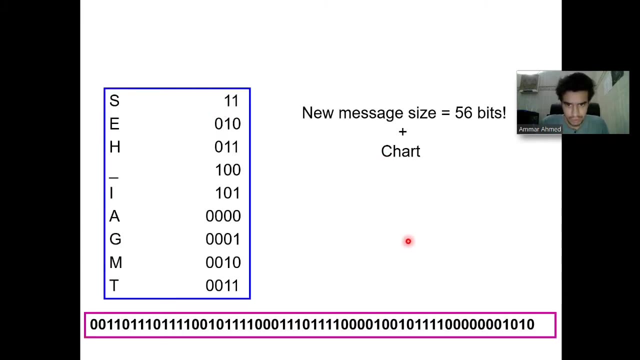 traverse to the left, append 0. whenever you traverse to the right, append just something after one. whenever you traverse to the right, append one. so, essentially, H has a code of 0, 1, 1 rather than 8 bits, right? so this is the new sequence, right and you? 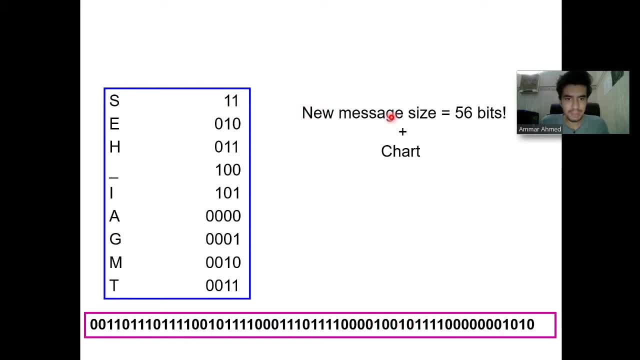 can see the size is reduced right and I've written here: new message size is 56 bits. but we also need a chart. what do we mean by chart this chart? so we have the sequence, but we don't know that which of these bits correspond to which character. 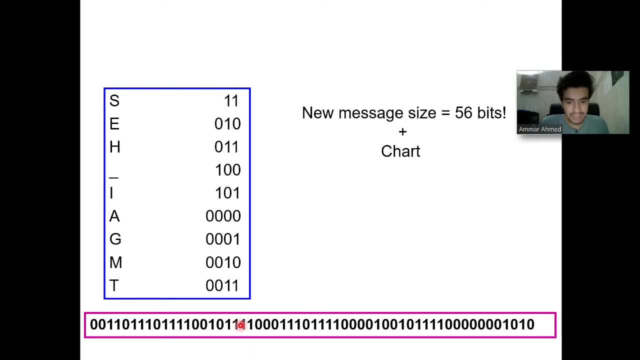 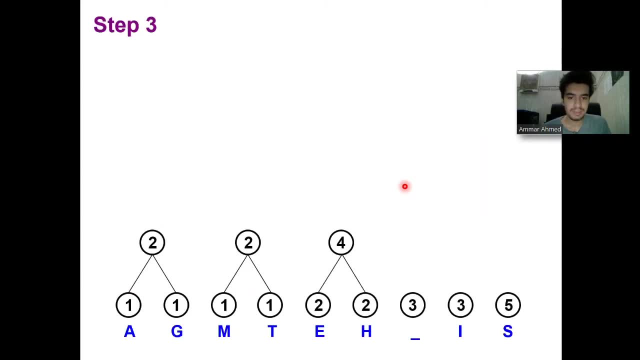 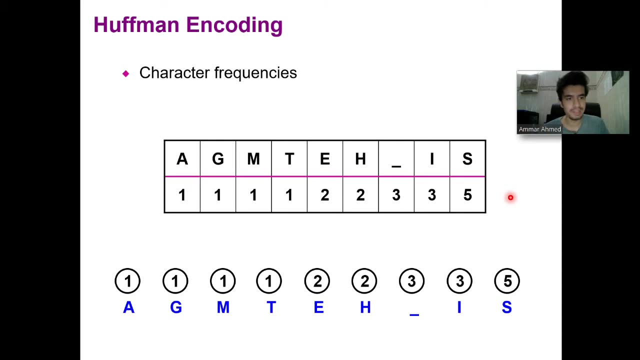 right. so we also need this chart and we also need this sequence. okay now, first of all, we need- I've told you that we need nodes, right? in other words, I also need frequency of each character. given a file as an input, I can represent this file as a string, but I also need for each character, I need a frequency, right. 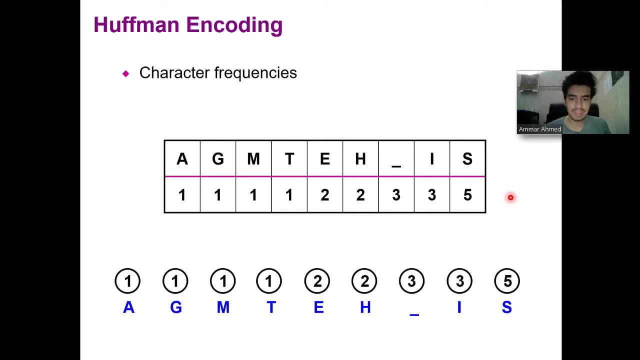 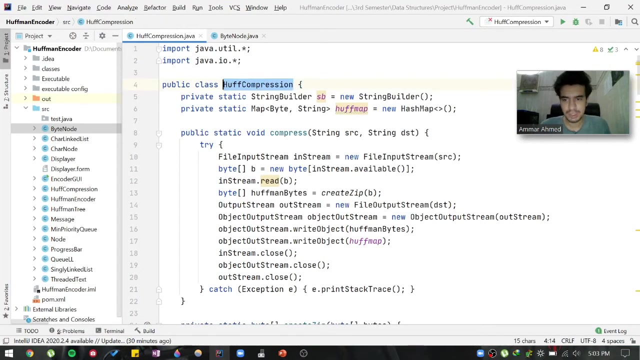 that's the first task that I need: to calculate the frequency. the next task is to convert these frequency and characters into nodes, right, and then somehow I have to select least two nodes and then combine them, right. so let's now look at the code, right? so I have a code here. this is the class called Huffman compression we have. 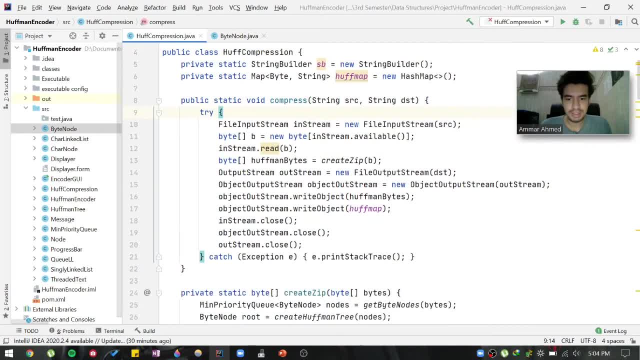 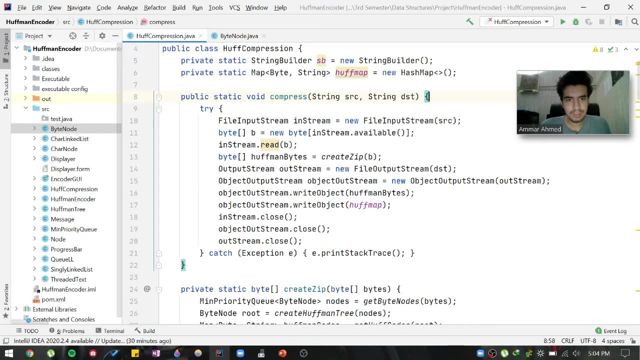 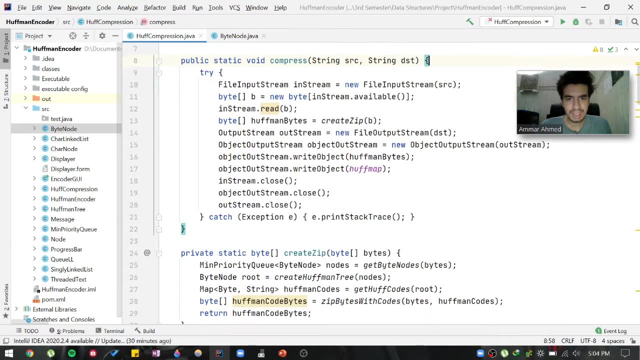 other classes as well, but this is really the class that does the compression and decompression business. so in the, you know, in the, in the method called compression, we are taking the source in the destination as string data types, right. and then I'm saying that, okay, I created this, you know, area of bytes, right in. 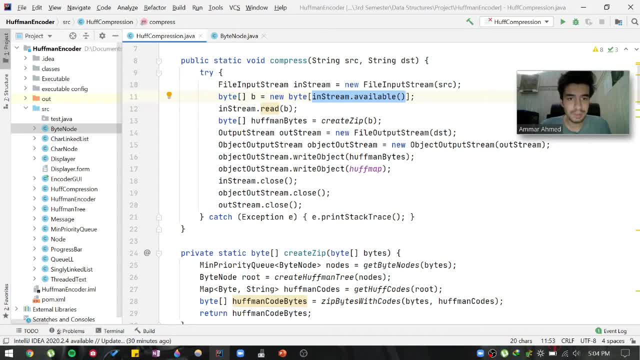 which the length of the byte is, how many ever bytes are available, and the given file as an input, and then I'm just reading all the bytes into this byte array. so the question here is: why am i, you know, reading bytes right instead of characters? well, if I read characters, 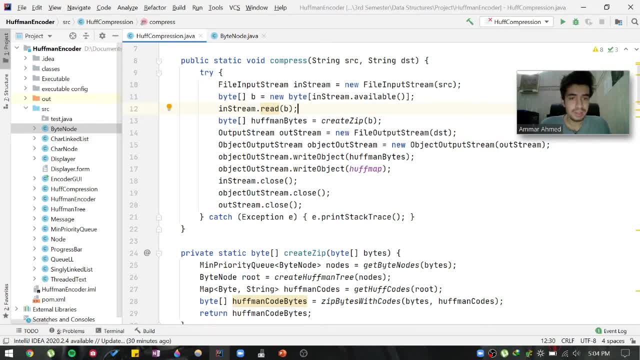 then the size of the you know compressed message is going to be, you know, increased. so I don't want to increase the size rather than I want to decrease the size. so we have decided to use the byte representation of each character rather than the character data type itself. okay, after. 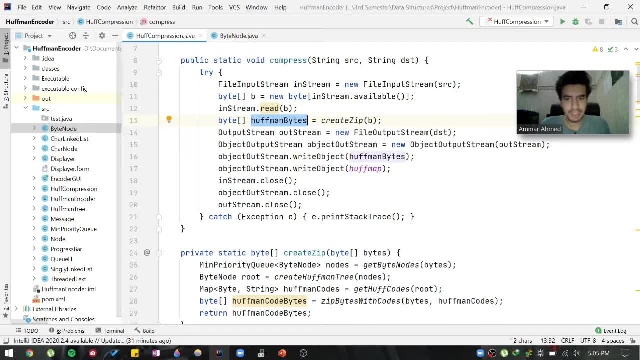 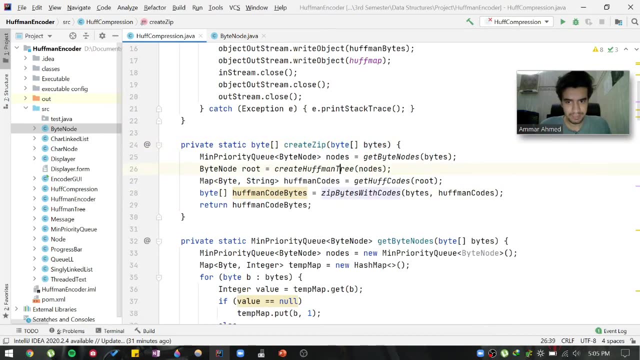 I've done that. I'm creating the area of type byte in which I'm calling- the method creates it- in which I'm passing the this area which contains all the original bytes in the file. so what this clear zip is going to do is it's going to take the byte array and then it's going. 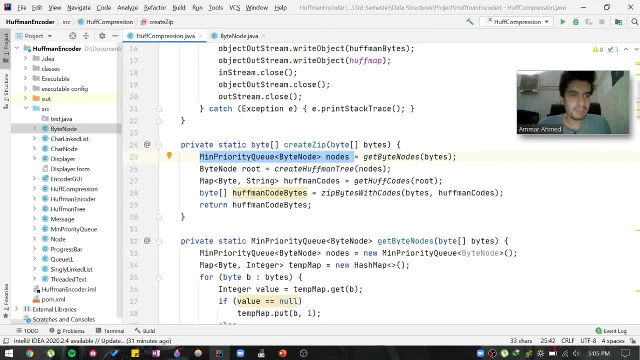 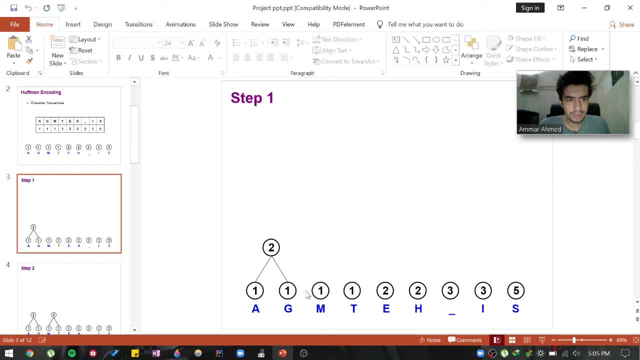 to create a minimum priority queue, right? so why are we creating a minimum priority queue? if you remember, I've told you that each time we have to select two nodes with least frequency in this behavior. you know how can we achieve this behavior? the way we can achieve this behavior is by 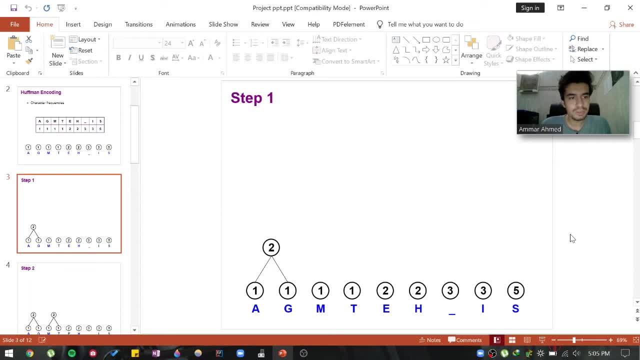 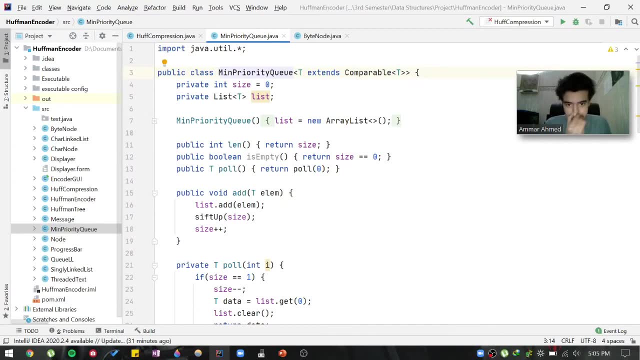 selecting the number of nodes in the list and then, by selecting the number of nodes in the list, use min binary heap or min priority queue right. so we have implemented min priority queue. you can see this class min priority queue, in which we have used min binary heap to add and pull elements. 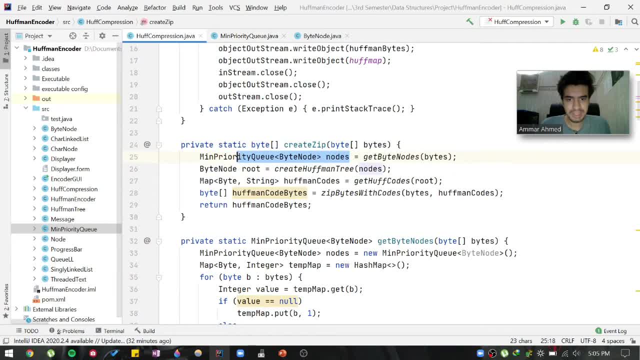 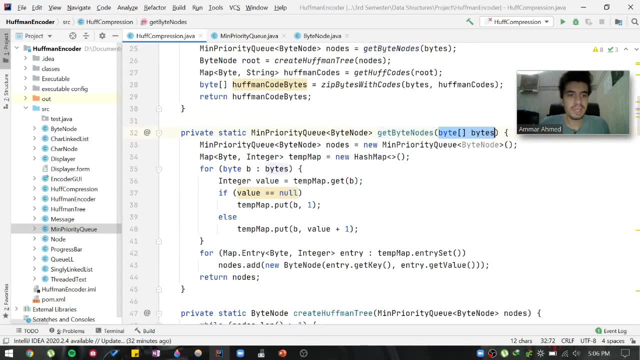 right. so I've just essentially created this min priority queue and I'm calling the method get byte nodes. and what this get byte nodes method is going to do is that it's going to accept the original bytes and then it's going to create a new min priority queue and then 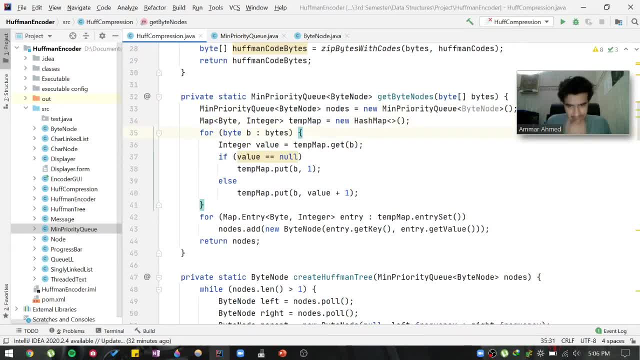 it's going to create a hash map, and what this is going to do this for loop is that for each byte, in other words, for each character, I have to calculate its frequency. so this is exactly what I'm doing here, right? so I'm creating an integer value, right, in which 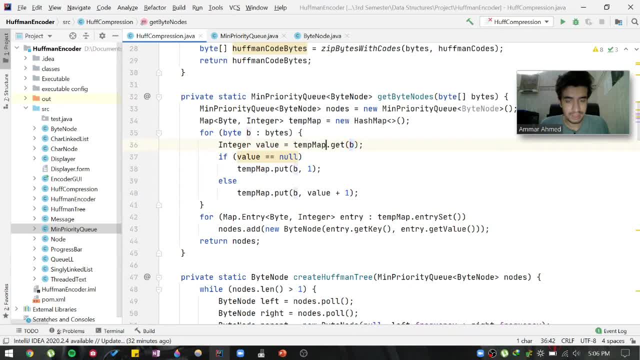 I'm passing the byte, in other words a character, and I'm saying ok, if the value is null. in other words, character had never appeared. it didn't appear, looks like it says a and then let's is, for example, more than one time. just put this character with the frequency of 1. 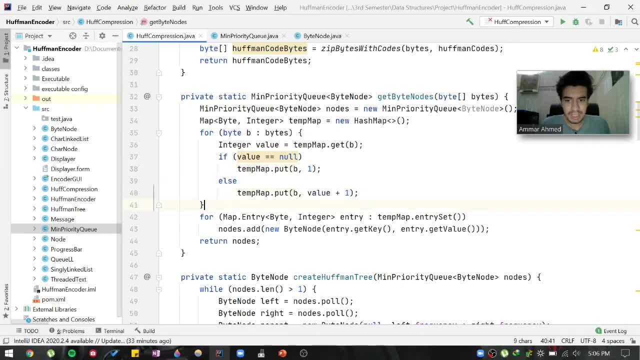 otherwise increment the frequency. right after I'm out of this loop, I'm doing a for loop. I'm just. what I'm doing here is that I'm adding a node, right? this is exactly what I was talking about. I have to create these nodes in which I'm 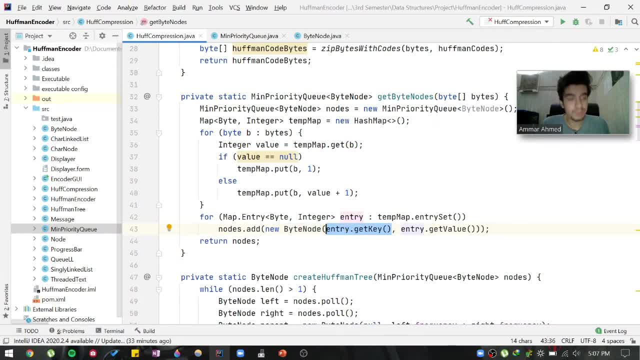 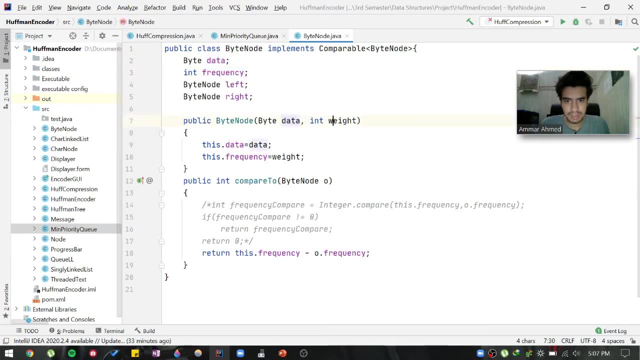 passing the gate key, in other words, the character itself, the byte and the value. and what is the value? value is the frequency of a character. so if we think about the byte node class, I'm accepting data in frequency right in this constructor. okay, so this is all this method is going to do. okay, so we. 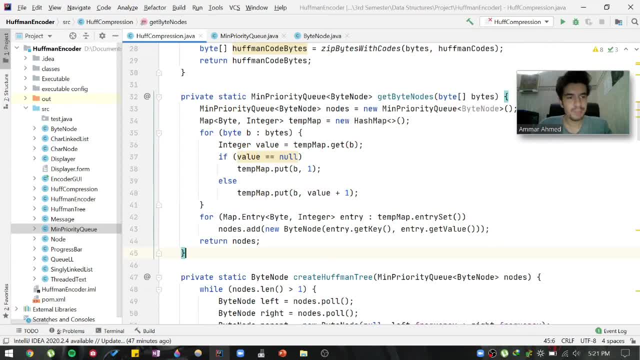 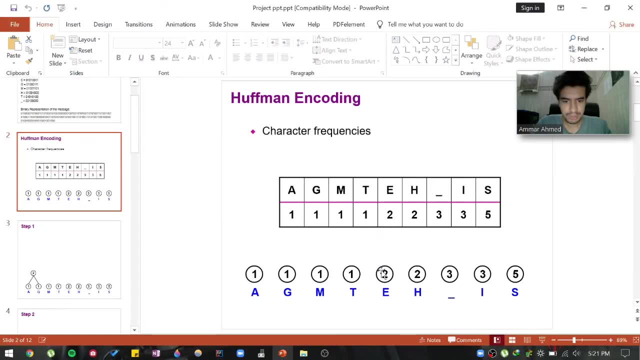 have calculated the frequencies right and we have created a min periodi queue right. so two tasks are done. we have created. so we have created the nodes right. we created the nodes with character and their respective frequencies and we have also calculated their frequencies right. so these were the two tasks. like I said, that I'm 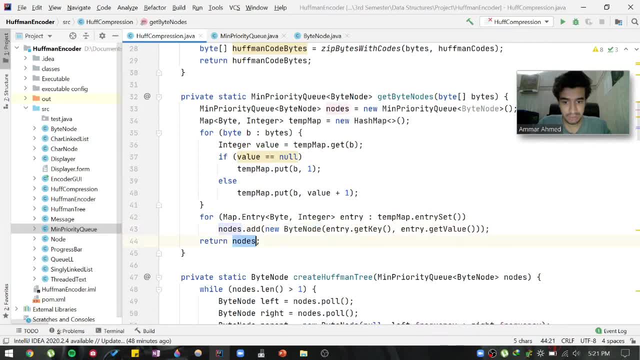 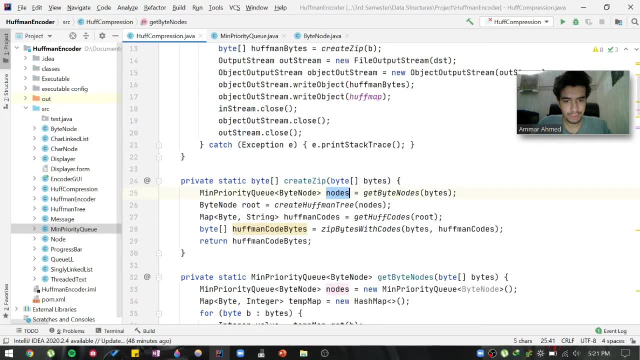 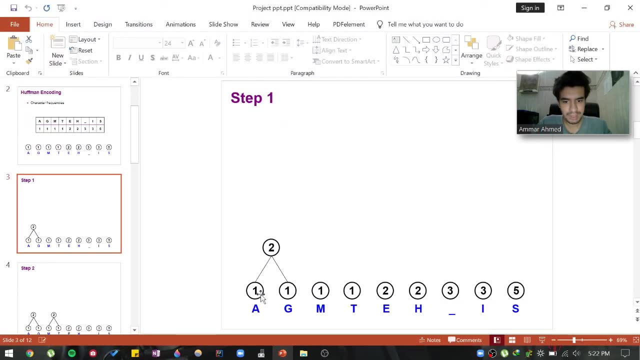 adding each node into this min priority queue and I'm just returning this min priority queue containing all the nodes of distinct characters with their frequencies. so this min priority queue is going to be assigned here. the next step is to build a tree. right, that is exactly what we are doing here. after, 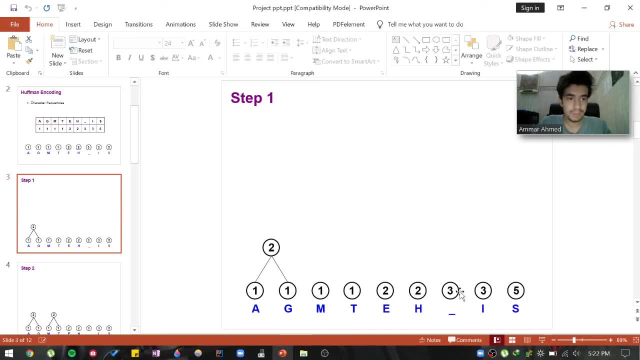 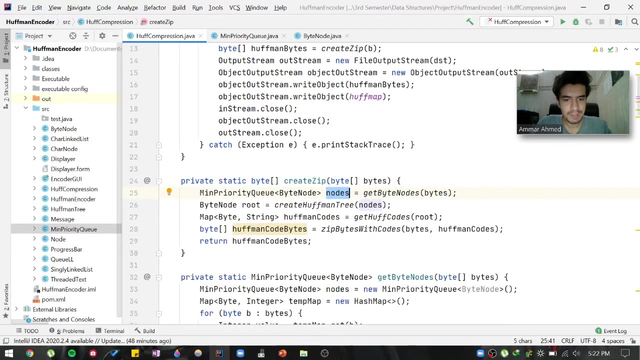 creating all these nodes. I have to somehow create a Huffman tree by pulling the least two nodes out of the min priority queue and creating another node, the parent node, in which you have these two children and its frequency is the sum of these two nodes, right? how can we achieve this? so I'm creating a byte node. 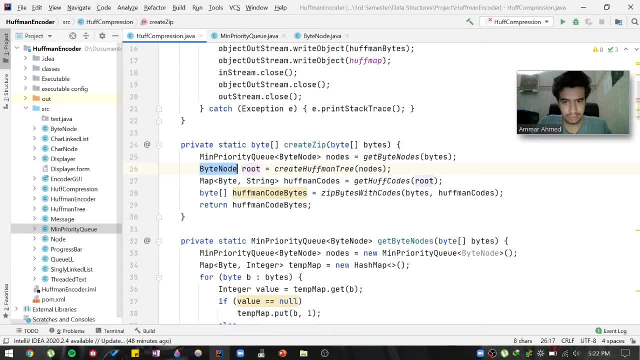 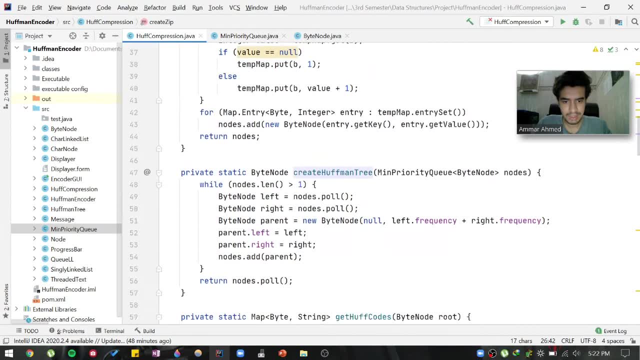 of type. you know root of type, byte node right. and then I'm going to create a min priority queue and I'm going to create a minute loop and then I'm going to create a minute loop and I'm initializing whatever. this is going to return right. so create Huffman tree. is this method? 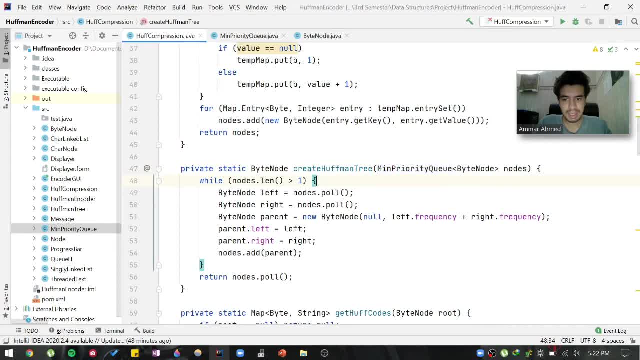 here and it's going to accept a minimum priority queue that we have just created, and it's going to run a loop while the length of min priority queue is greater than 1, right. so right now I'm pulling the two least elements, so here we can. 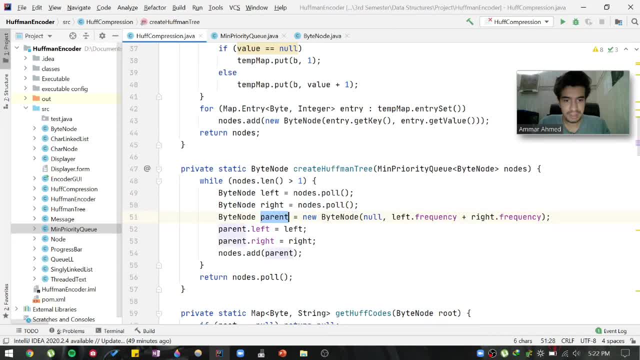 see, I'm pulling the least two nodes and then I'm creating a new node, parent and parent, in which I'm passing the frequency as the sum of these two nodes and this is just null, because I don't want to pass any character, because I don't want to represent this node having any character, and 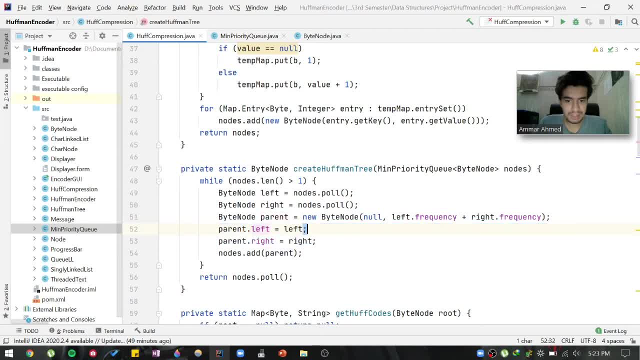 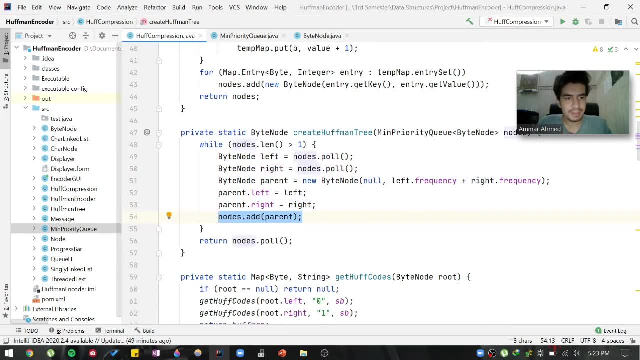 I'm just, you know, setting parents left is left and right is right, in other words, this, these two nodes, And then I'm just adding This parent right. so these two nodes have been pulled. so in other words, They are removed, right, But I've added this parent right which is the parent of these two nodes. so so somehow you can see in. 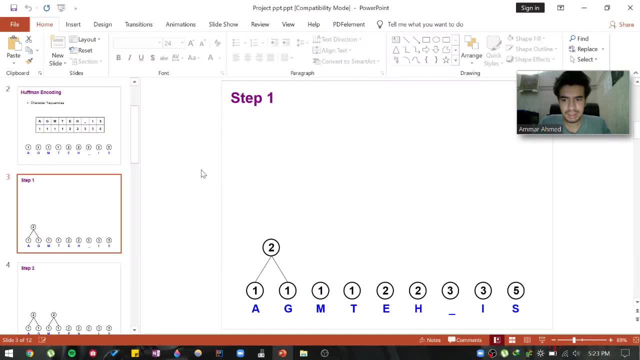 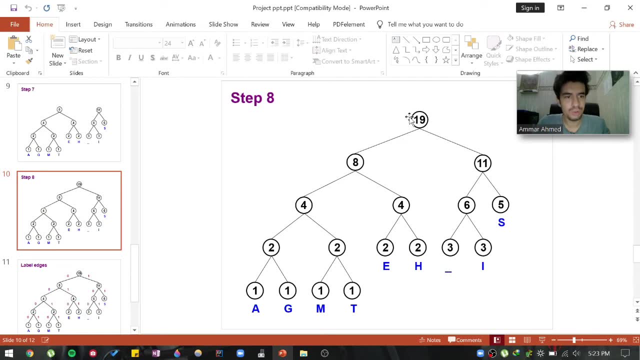 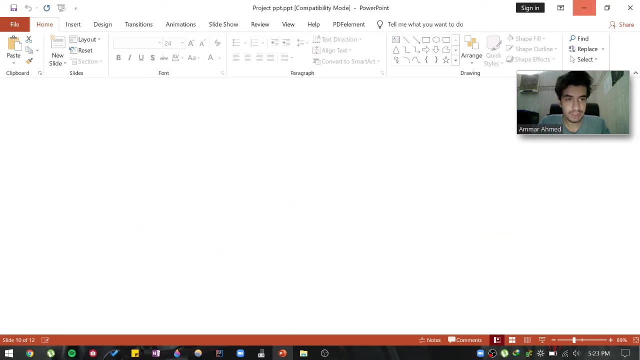 the process there is going to be Only one node left right in this min priority cube that is going to be 19, In other words, the root node that contains all these nodes, right, including These nodes that have characters and their frequencies, right. so in the last I'm just going to return this root. 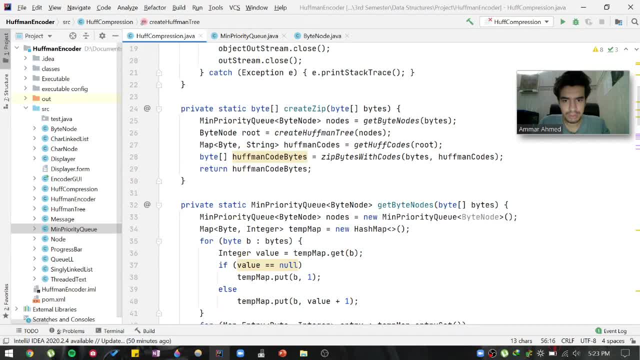 By pulling this element. This root is going to be assigned here. okay, Next what I'm doing. so what is left now? We have created the Huffman tree, We have calculated the frequencies, We have created the min priority queue. The next step is to traverse the tree and get the new codes right, instead of 8 bits that we were. 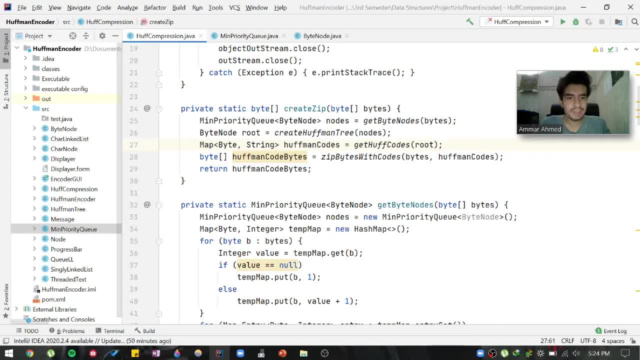 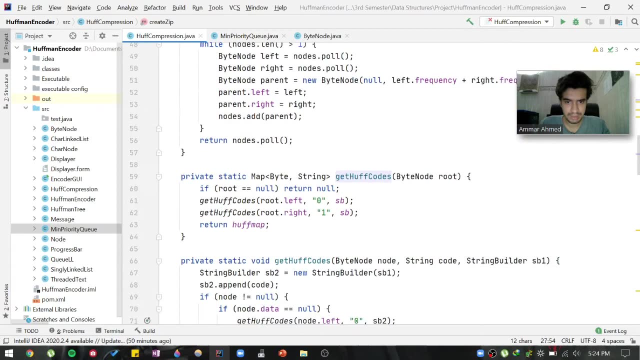 Presented with. initially now we are going to get the nice sequence of each character. so this method here. So I'm creating a hash map called Huffman codes and then I'm calling this method: get Huff codes by passing in the root right. So this method right here is going to do nothing. This is just a recursive method in which I'm 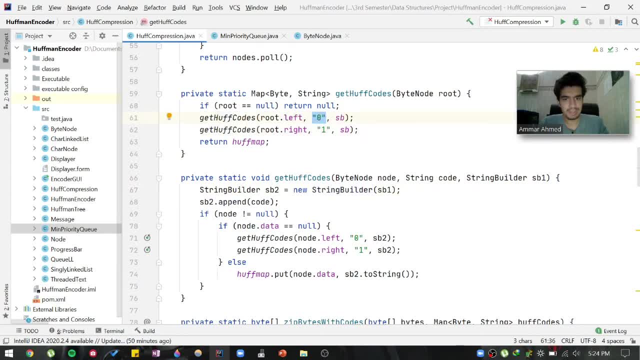 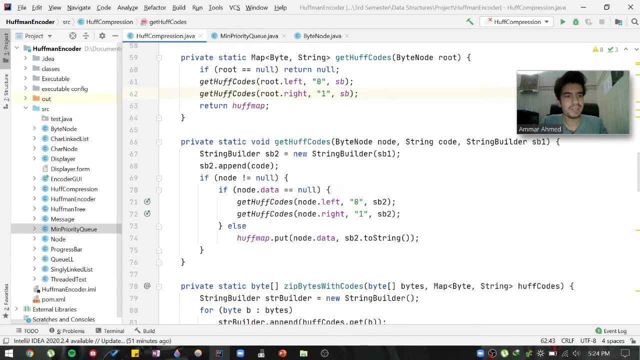 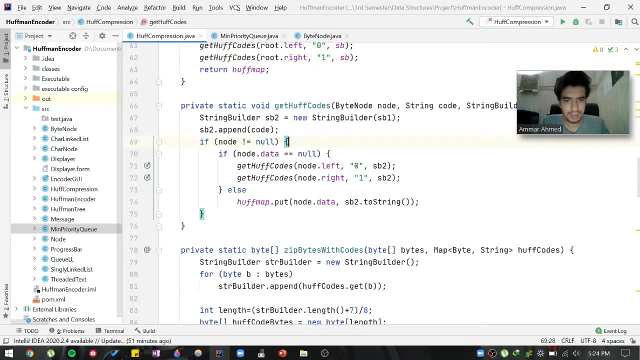 Passing root dot left with initially 0 is a string in a string builder. right, you're going to see what this string builder is going to do, because Why am I creating a string builder? because I want to append the Sequence in a string, right? so here, all I'm doing is that, okay. 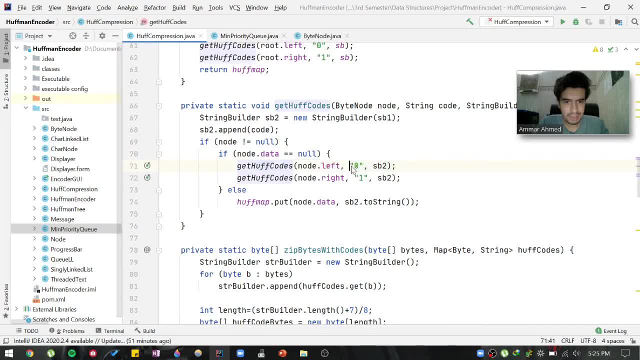 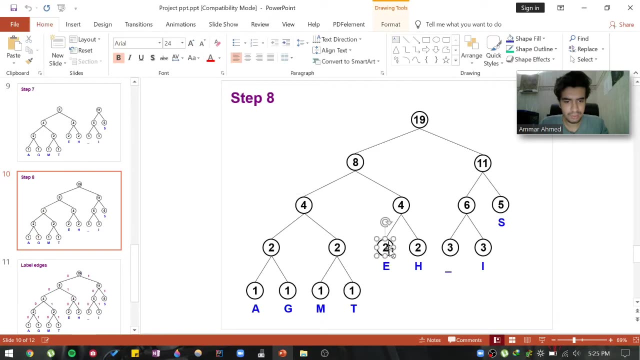 If I traverse to the left, Just append 0. if I traverse to the right, append 1 right. so if You are hitting a leaf node, right. in other words, if you, if you somehow get to this node, This, this, this, this or this, any of these leaf nodes, that means I have to put 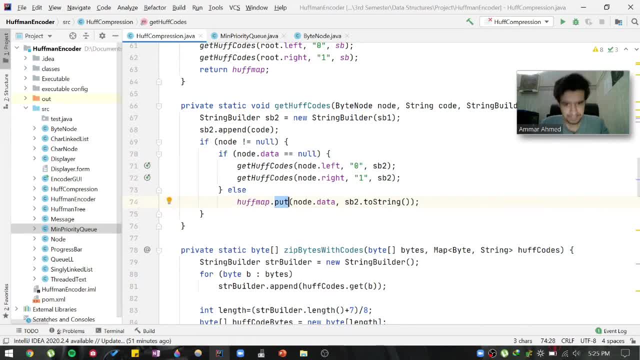 this. What do you call node? It's data. What do you mean by data? data means the character and its sequence right. so in the Huffman right I'm just going to put the character and its sequence right. so, in other words, if I want to, if I hit this node, suppose a 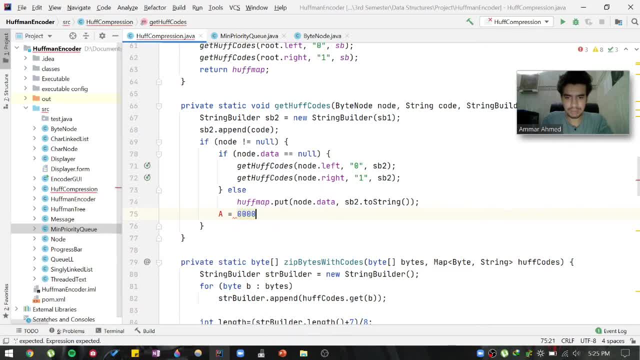 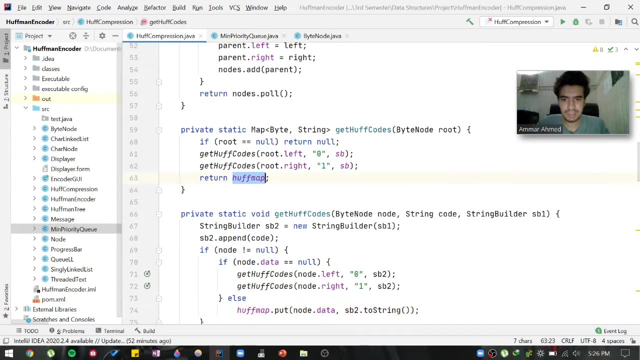 It's. This will be zero, zero, zero, right? so what this is Going to do is that it's going to put a here and also the sequence of The character, this new sequence. right, that's all I'm doing, and in the end, I'm just returning a Huffman that is going to be initialized this: 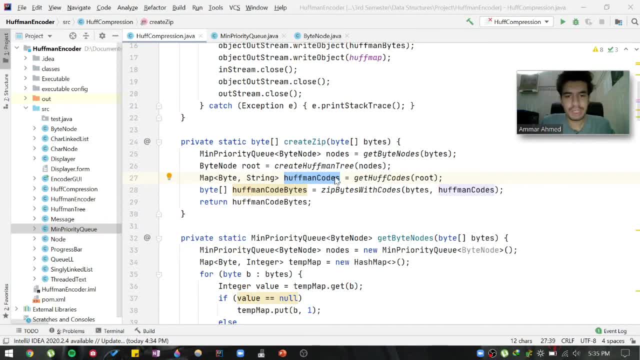 Huffman course. right, Okay, so now that we have this Huffman course, This is a hash map containing the characters in the new sequence. right, the new sequence, meaning that After we have traversed the whole tree, we have now a hash map for each character. you have a new sequence now. 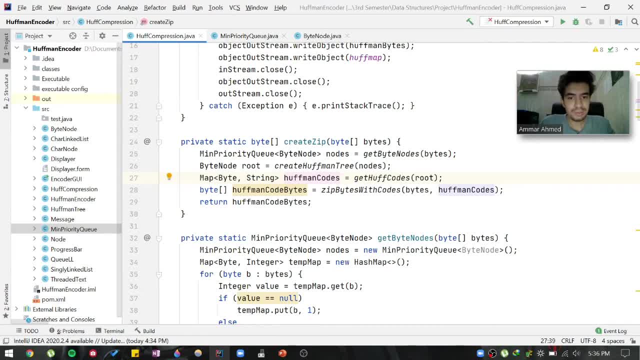 What is next? The next step is to store this new sequence in a file so that we can read it back right to decompress it. So somehow we have to store this sequence, in other words, this hash map, Right into a file. So this is like a chart that I was talking about. right, you have to look at the chart and 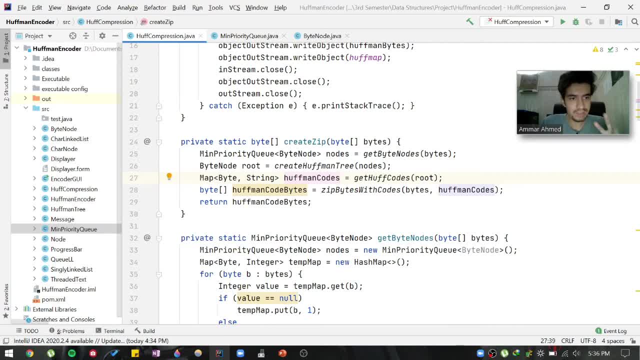 Then decompress the sequence. in other words, we need to store two things. We need to store the sequence, We need to store this chart, In other words, this hash map. so I am storing objects here. first I'm going to store the object of this, this hash map, and 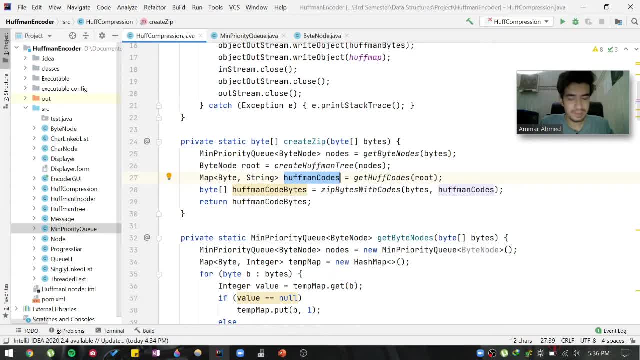 Also, I'm restoring the object of byte array, So you're gonna look at it. We're gonna look at this method: zip bytes. with course, This is going to do nothing, just Return the. it just returns the byte array which is going to be initialized here. So let's look at this method. 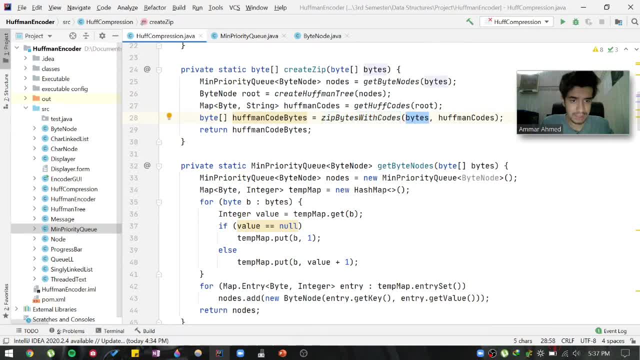 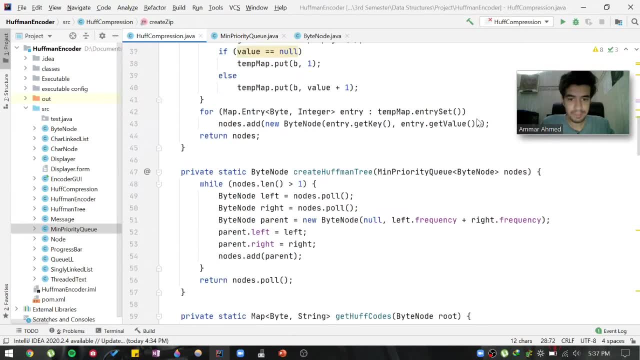 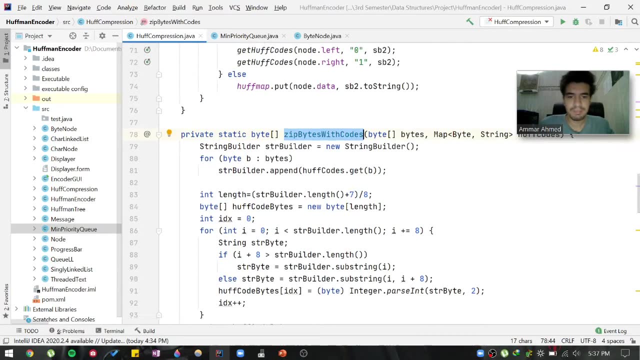 In which, remember, I'm passing the original bytes in this new hash method that we have just created, in in which we have characters And it's a new sequence. okay, so when we go to The zip files, with course, right. so zip bytes with codes. 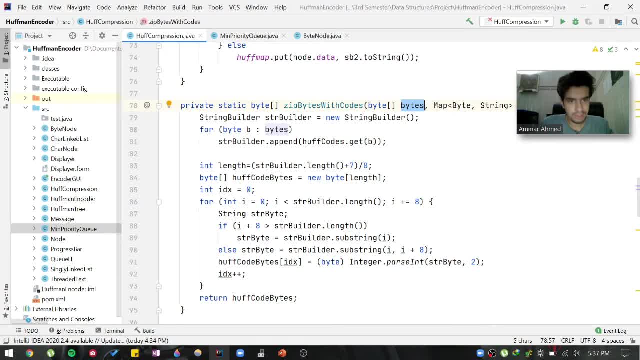 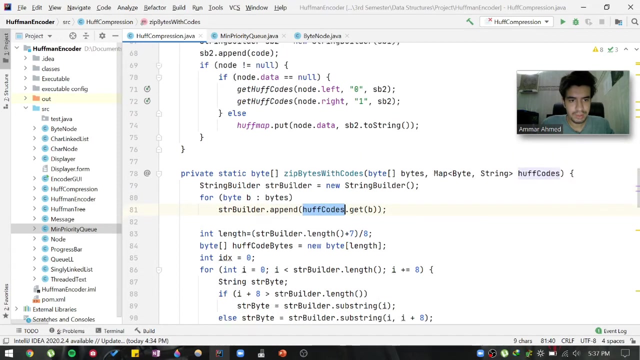 having the original, All the original bytes, it's going to run a for loop, right, and it's going to append the new sequence for each character, right. So it's going to get what you call Character right and it's going to append The New sequence, right. So what is half code, right? half code is a hash map that we have just passed, So 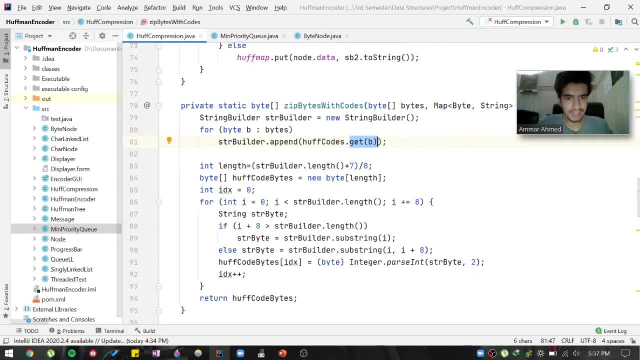 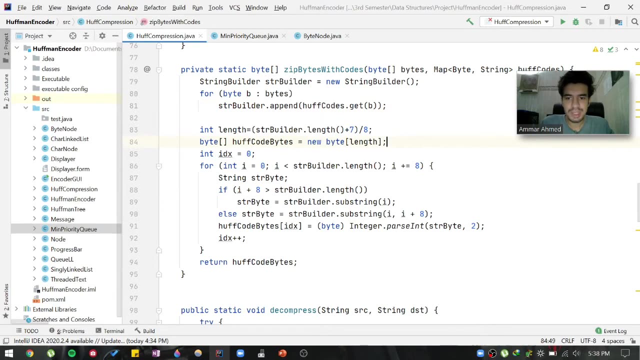 Obviously, when I call this method, dot get B, It's going to Scan the hash table, right the hash map, and going to return the string sequence. So it's going to be a painted in a string builder. Next, what I'm doing is I'm going to create a byte code, half code bytes, in which I am: 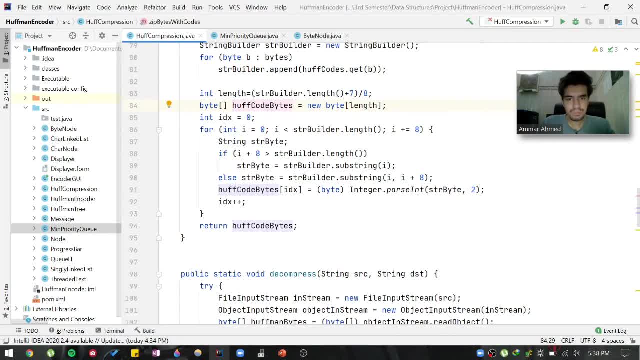 storing What you call The group of eight bits. So, given this sequence that I've just appended, I'm you know you're cutting this into eight groups, right? This is. this is the loop. I am pages C: I'm looking at tess's nicely ping where nfc and this line in the pode. 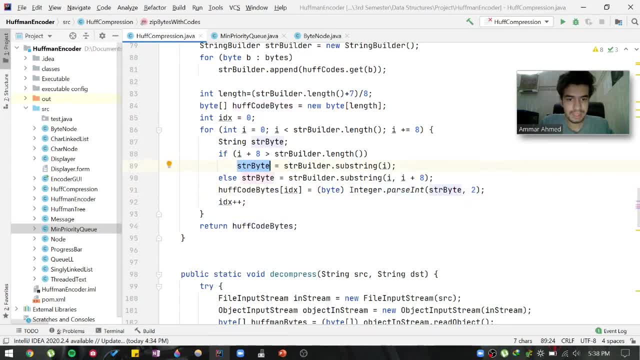 So you can see this essentially: first of all I'm painting it to it string and then I'm Parsing this string into integer and then finally making it a byte and store it into a half code bites and then return this half code byte id when this is returned. 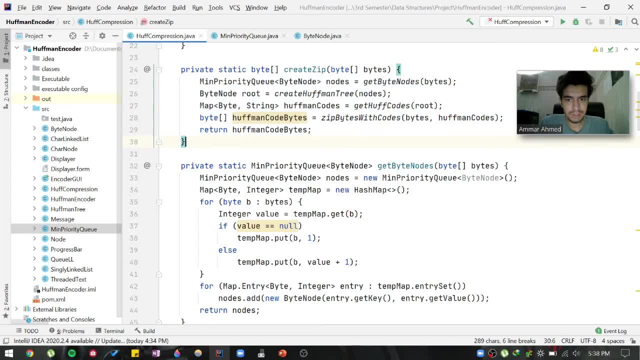 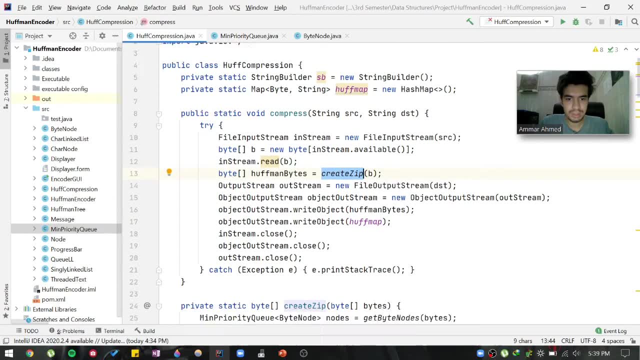 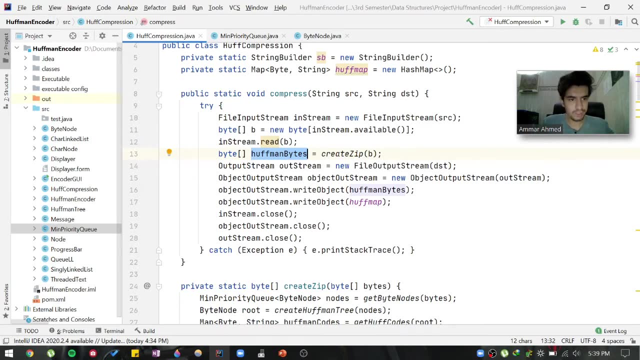 right, it's initialized to this and this is returned back. and when we go to the when this method was called, this method is just going to be returned. right, it's going to return this Huffman bytes, in which you have all these compressed bytes, in other words, the new sequences. I'm just going to now create output stream and object output stream, and. 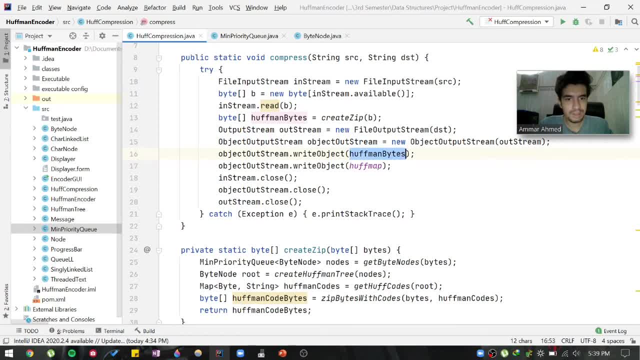 I'm going to do nothing but write the object: Huffman bytes, this compressed by: and Huffman Huff map. what is Huff map? it is a hash map that we have created in we have, in which we have character and it's new sequence. right, that's all we have done here, right? okay, so we've. 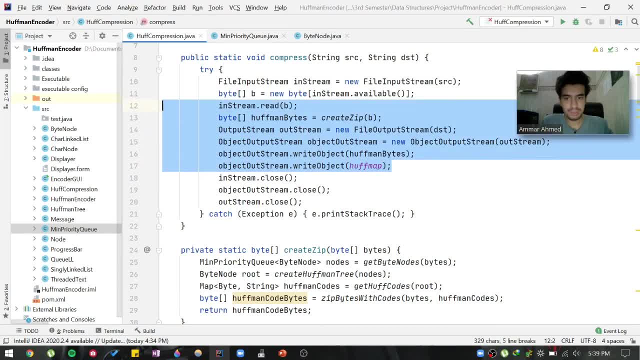 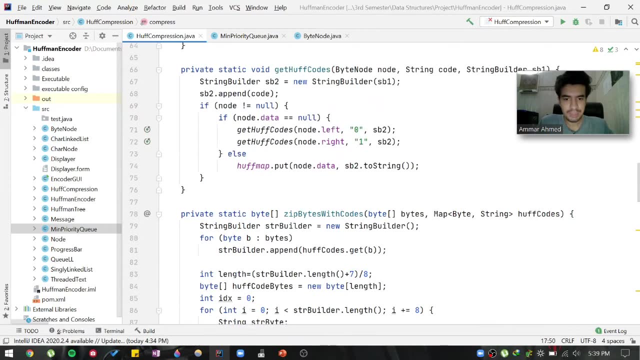 essentially done: the compression right. so this, this is the process of compression right. the compressed file is going to have two objects that will have size significantly reduced- right. but now we have to do decompression right for decompression. I'm doing nothing, I'm just doing the same process, but in reverse right. 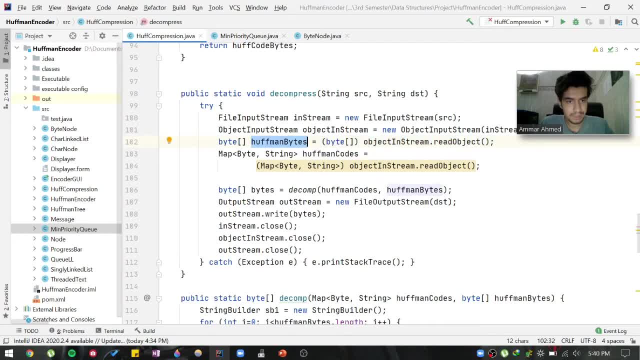 I am reading the object of Huffman bytes that we have stored. I've just told you that we've stored two objects. one is the array of byte, of type byte, and we have stored hash map right. so I'm just reading the byte object and I'm also reading the hash map object and initializing. 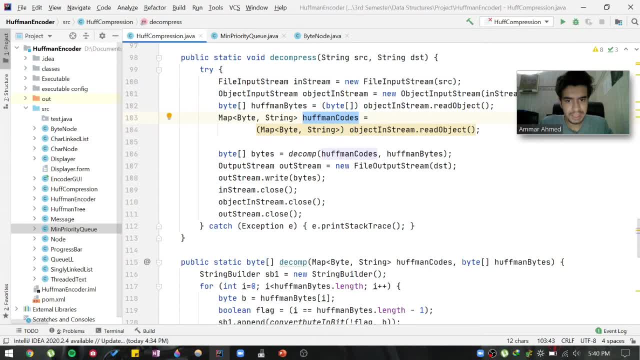 them to Huffman bytes and Huffman codes respectively. and then I'm calling this method decomp, which is going to return the original bytes, right. it's going to decompress these Huffman bytes, right, using this chart, using this hash map, and it's going to return it and initialize it to bytes. and then I'm doing nothing, I'm just writing the. 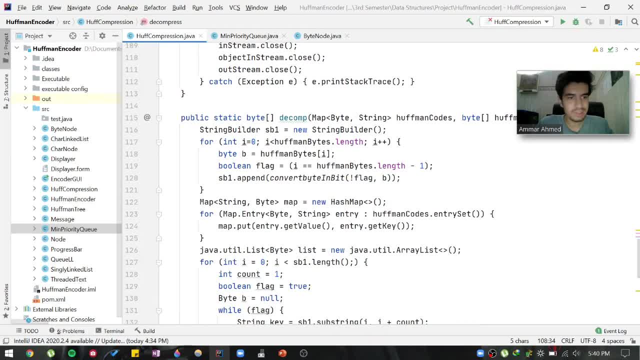 original bytes back, essentially decompressing the file. so let's just look at the decomp method. so finally, we have to discuss the decomp method. so decomp method is doing a simple job. it's just doing the reverse process that we have done. so it's. 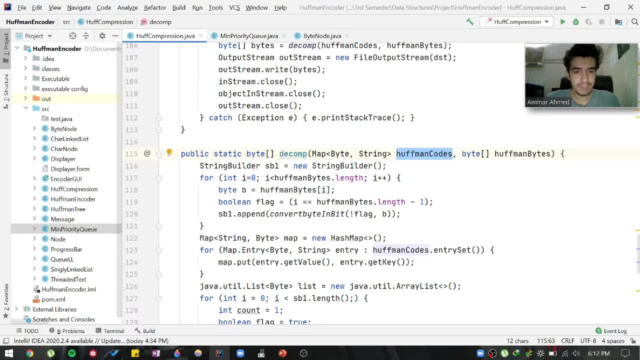 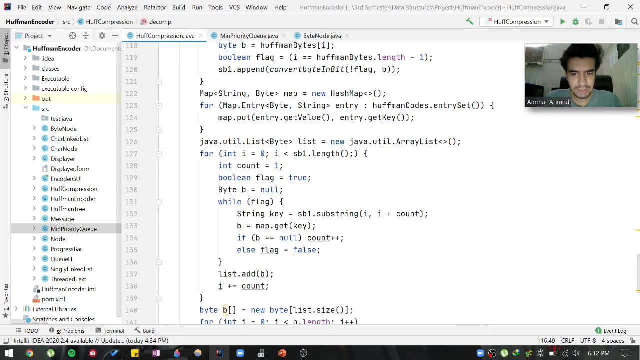 going to take the bytes and the hash map that we just read from the compressed file and the Huffman bytes, right, the compressed bytes, in other words, group of 8 bits. so this is going to do the reverse process, right? so, in other words, I'm making a map and then, for each string key, I'm then just going. 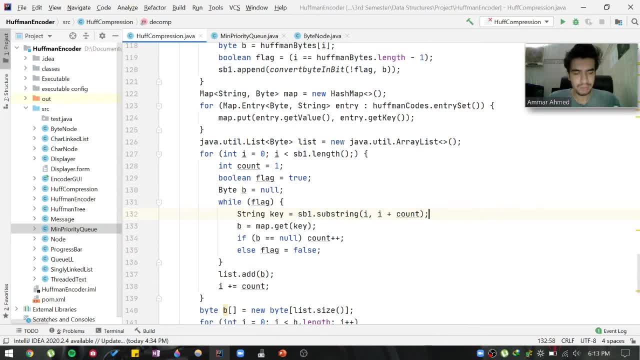 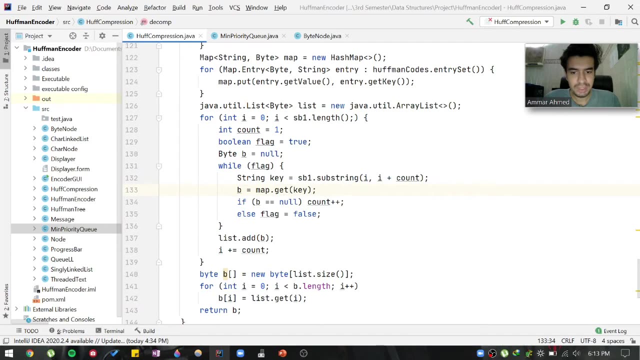 to take what you call I'm so, for example, from 8 bits, I'm going to look at the sequences of each characters and then I'm just going to return the key and then I'm going to get the byte from each of this key right. so after doing that, I'm 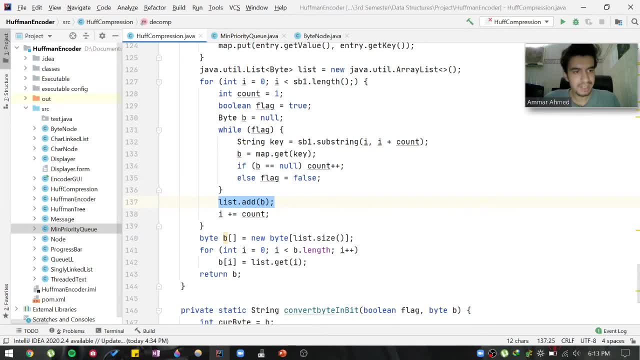 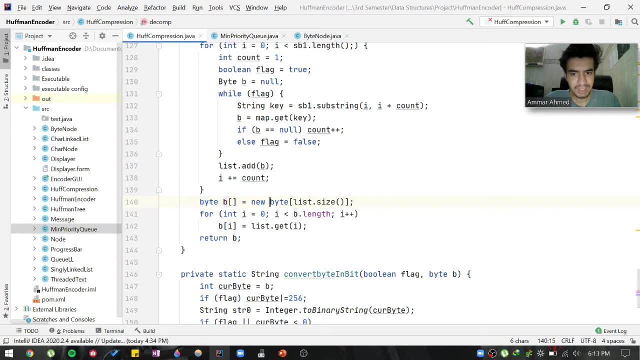 just adding it to the array list, right, and after adding it to the array list, when I come out of this loop, I'm just adding this- all the items in the array list- back into this byte array. so now this byte array now contains all the original bits that we started with right, and then I'm just going to. 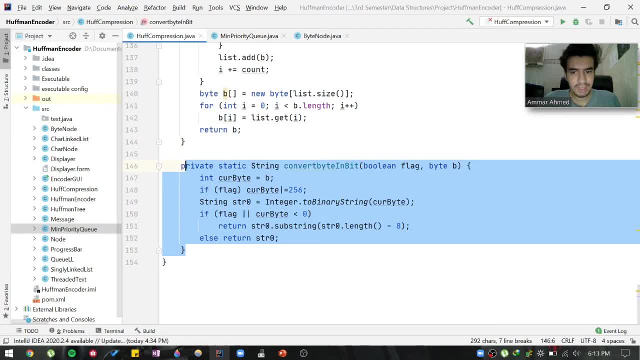 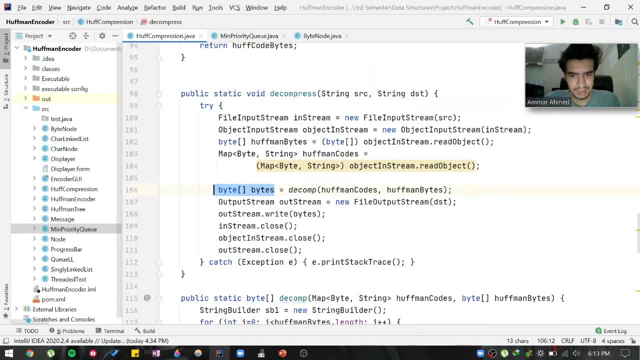 return this P, right? so this is a helper method to convert into a bit. so this is going to return a string, right? so this byte array is going to be initialized with the original bytes that we started with, and then I'm just creating an output stream and then 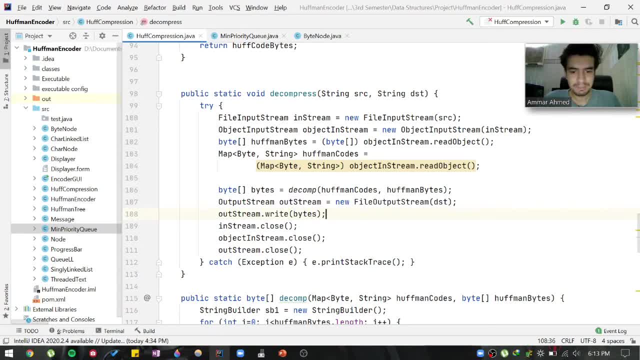 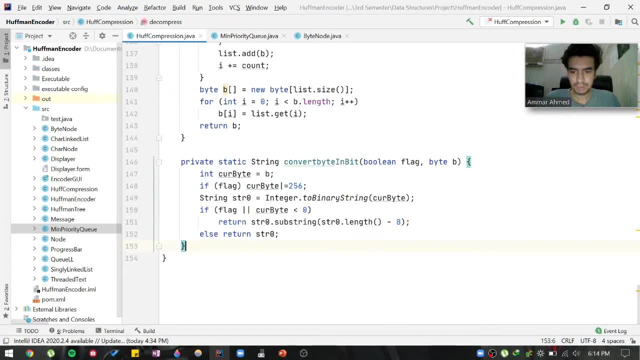 writing the bytes back into the destination provided. so let's just look at the working of this whole code, right? so what I'm going to do here is I'm going to create a public main method, right? so these are stating methods, so I can access them. I'm going to call a compress method. I'm going to 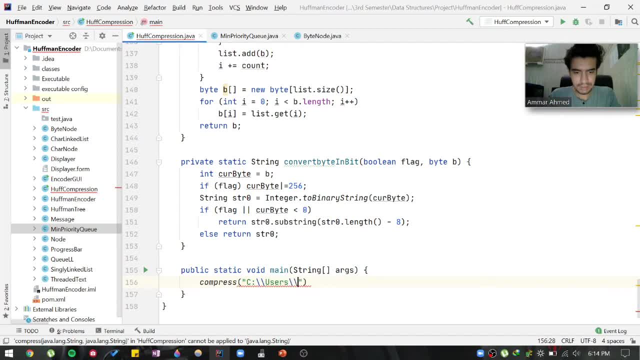 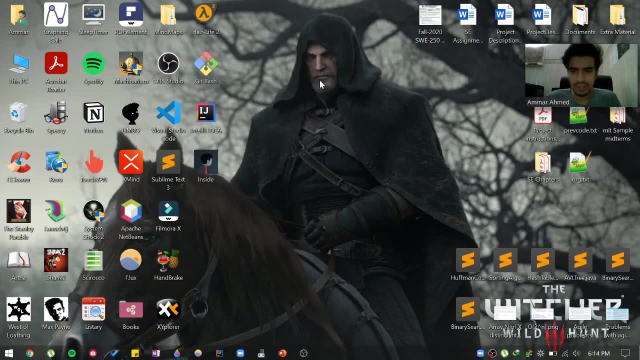 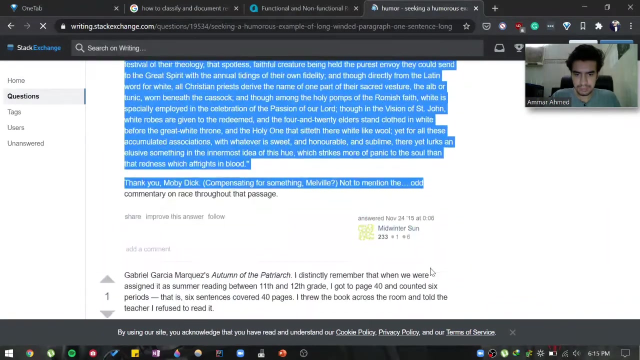 provide a destination. so, for example, I'm going to provide it a desktop, and let's say I want to compress a text file. let's say I will call it text and let's just take any paragraph from. so I'm just going to copy this, right, and then I'm just 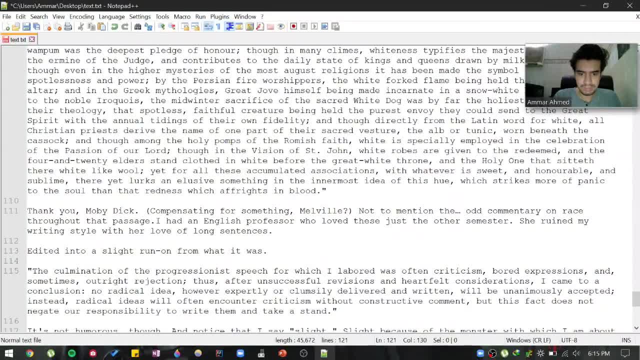 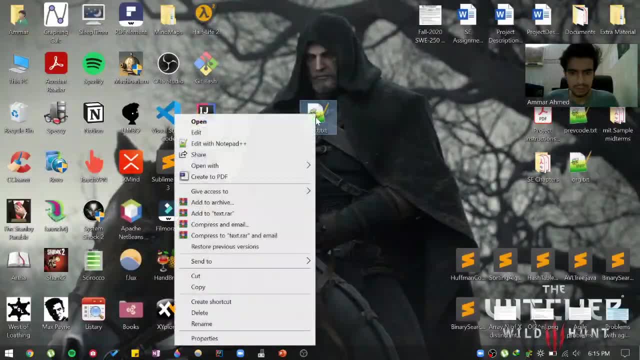 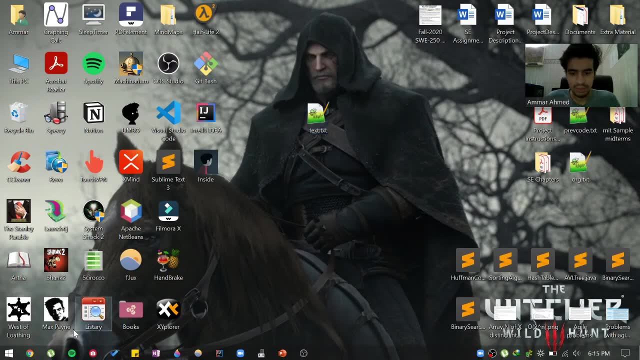 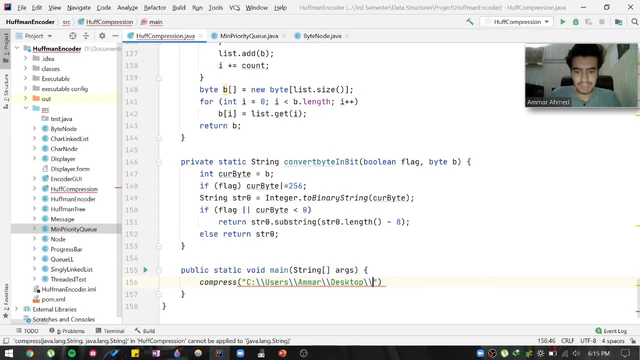 going to paste it multiple times to increase the- you know, length of the what do you call the file? so let's just look at the file size. right now is 446 kilobytes, right? so let's just see if we can compress this file and then decompress it pack. so let's go to intelligent again and let's 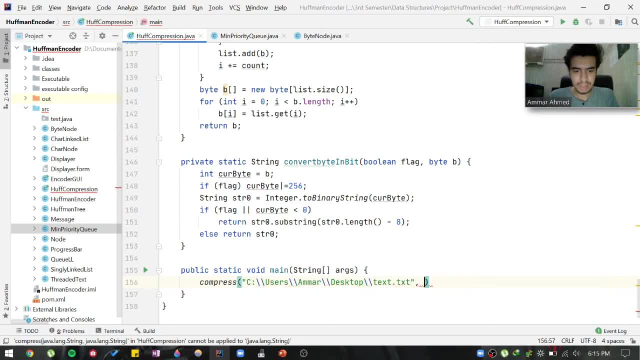 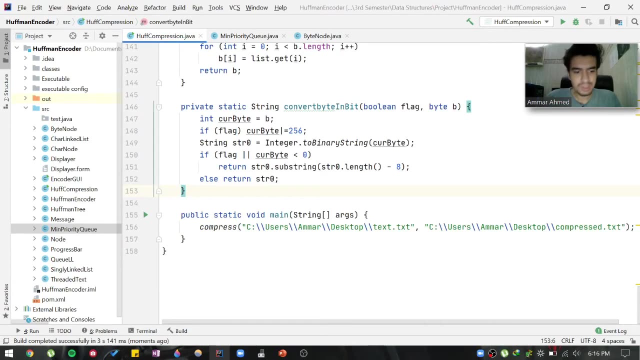 provide it a source and then also provide, when you'll call the destination right, so I'll say compressed right dot txt. so if I now run this man matter, right now that I provided a source and I have provided a psychedelic medium I have, now that I have provided a source, now that I have proposed. a Jericho have contains moreичего and they are going to complete four minutes. has to be so that they have complete four months, chapter one and I'll say paste. this is the check line. this is not thatGr hakkbb. yes, on the left hand side I'm basically have more businesses are fairly. not like context and managing the others and that is why all of my Deals with them was a two wheeler, but world dealing in order to do everything: rơv lizardconfigured, and I'm trying to make sure it's not the system. that's the reason. that is why I have 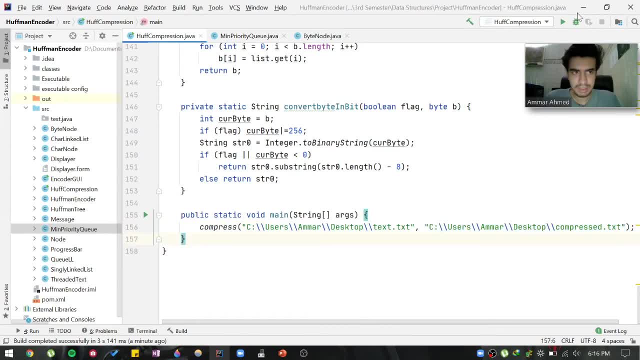 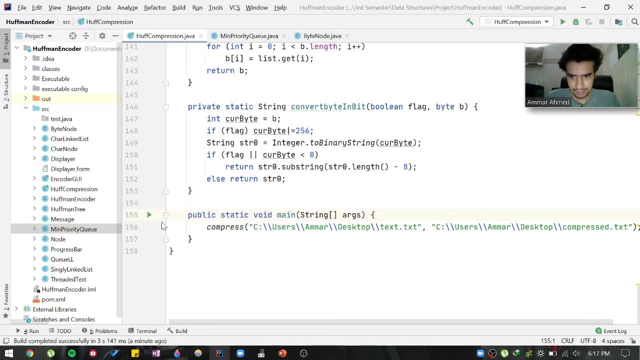 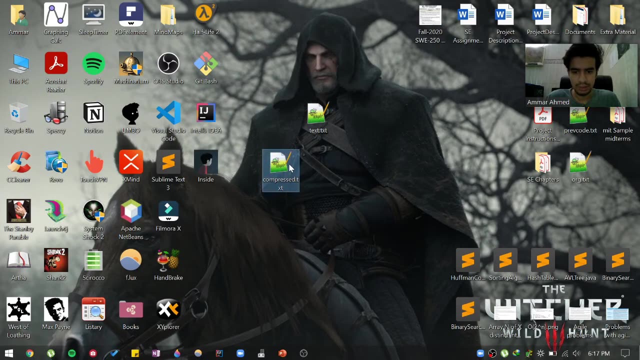 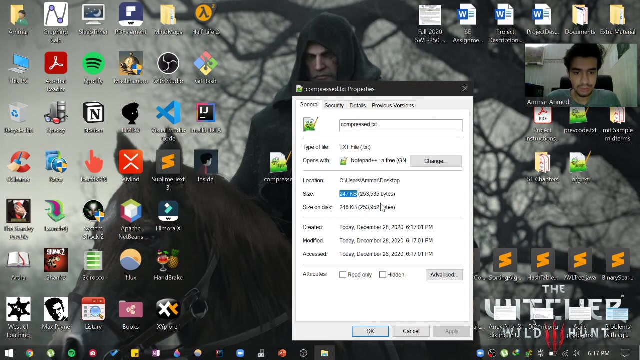 a sample right, and this file is here. let's just say, now i want to compress this file, right? if i run this program, the process is going to be finished and now you can see i have a new file called compressed. if i see its property, then the size of this compressed file is 247.